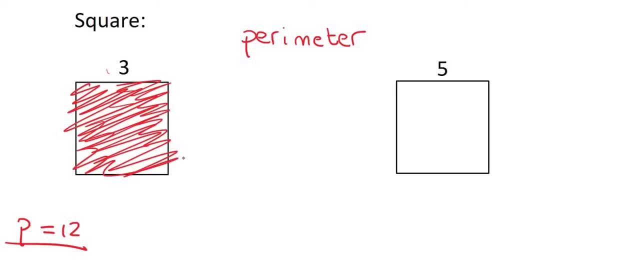 Okay, think about it. Think about what the word area means. If we're looking at a rugby field, for example, you could say that the rugby field has a really large area. Okay. or maybe you're looking at a house and you can say that the lounge has a large floor area. So area is not on the 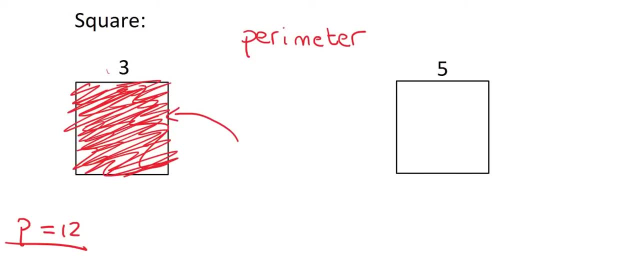 outside, it's all the stuff on the inside, And so how do we work out the area of a square? Well, let me show you exactly how this works. Okay, just for the first one. So we've got three units going for this length over here. So what I'm going to do is I'm going to make it three blocks. 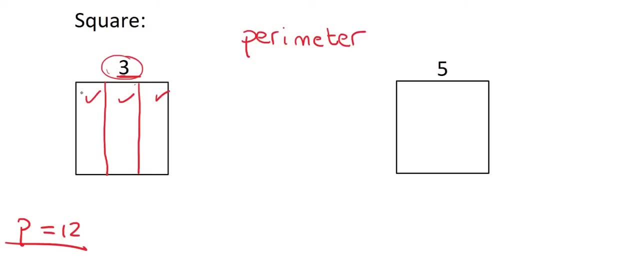 And so there you can see, I've made it one, two, three. Now I'm also going to do the same going down this side. I'm going to make it three blocks going across. What I then want you to do is count the number of blocks: One, two, three, four, five, six, seven, eight, nine Now. 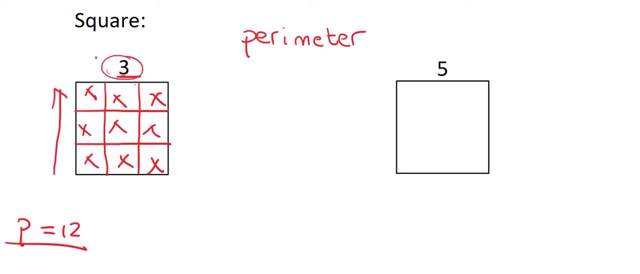 this makes sense: There's three rows going upwards and three rows going to the side. So to work out the total number of rows you could just multiply the three times three, Because, guys, you don't want to have to draw blocks like that, Maybe, like. 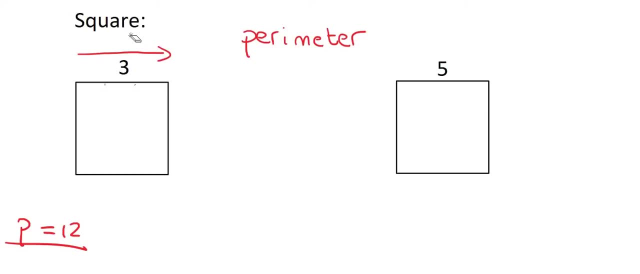 in grade three you could have done that, But in grade nine you don't want to have to draw blocks. It's not always going to work out so nicely, because sometimes they're going to give you a hundred as the length And now you can't sit in the exam and draw a hundred blocks. All right. 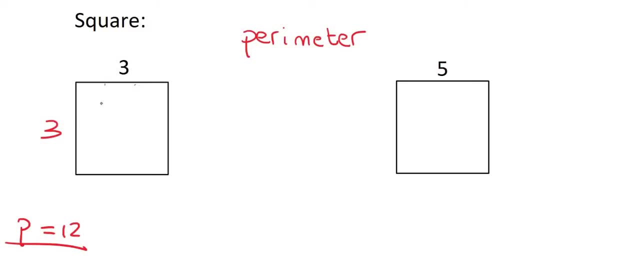 so if we know that this is three and three to work out the area which is all of this stuff for a square, you'll say three times three, And so the area is going to be nine. Now let's say that this was. I should have given us some units. Maybe this was in meters. then you'd say 12 meters over. 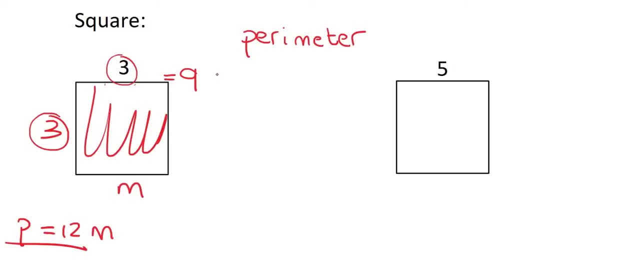 here, And for area you'd say 12 meters over here, And for area you'd say 12 meters over here. Because you're using, because you're multiplying two of them, you're going to say m to the power of two, So nine meters squared. So let's quickly try this one on the right To work out the. 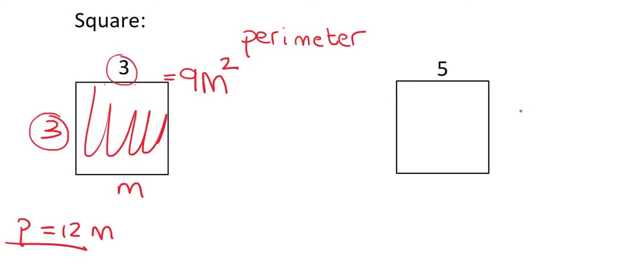 perimeter, you would just say five plus five plus five plus five, Or you could say five times four And that's going to give us 20 meters. Let's say that that's meters. Then for the area, we know that that's just going to be this, five times by this five, And so area is going to be. 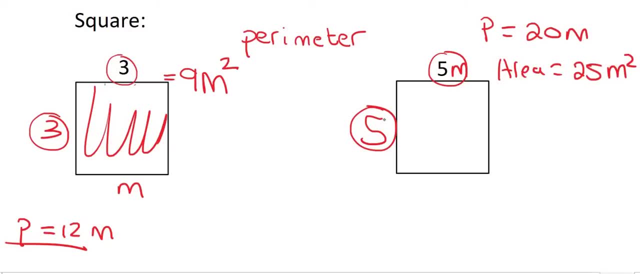 five times five, which is 25.. I know your teacher might give you these fancy formulas that you should use, but it's really good if you just understand what you are doing, So you don't have to memorize formulas the whole time. All right, moving on to a rectangle. So a rectangle is very similar to a. 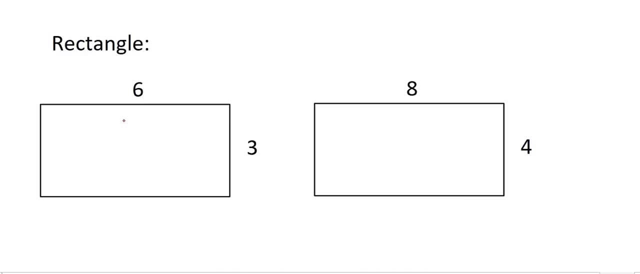 square, but not all of the sides are the same. But what we do know for a rectangle is that the opposite sides are the same. So this one will be six and this one will be three. And so to work out the perimeter, remember, you just add up all of the sides. So this one will be six and this one. 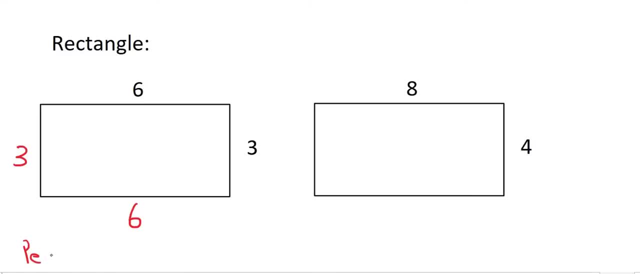 add all of the outside parts together, So the perimeter will be six plus six plus three plus three. Your teacher might say six times two plus three times two. The reason is is that there's two of these threes and there's two sixes. Okay, but you don't have to do it like that. You can. 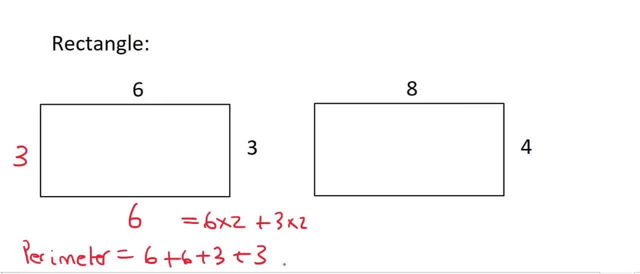 actually do it however you want, as long as you understand what you're doing. And that's going to give us 18 meters. Keep forgetting to write the units here, And then for the area, you can use the same approach as we did for the square, For example, if we have six units going. 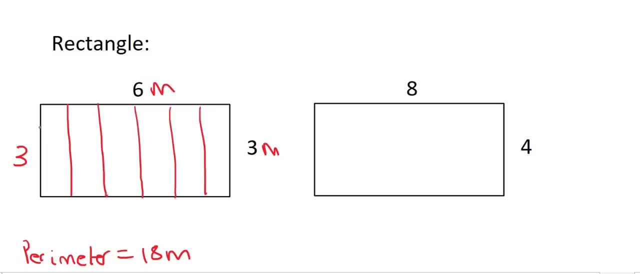 to the side. we can make six blocks. then we can make three rows going down And if you had to count the number of blocks, you would see that there is. just think about this carefully, guys, if you really, if you think about this carefully, how many are there at the top here there's 123456.. 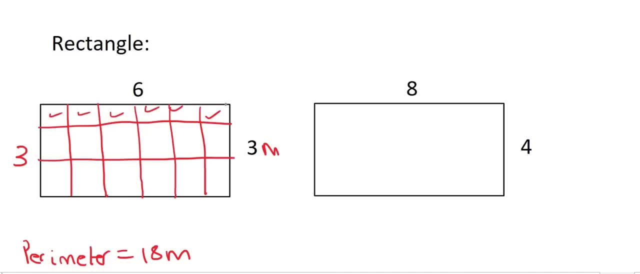 Now, how many of those rows are there going to be? there will be three of those rows, So we could say six times three, right. And so to find the area of a rectangle, you just say this number multiplied by this number, And so the area would be six times three, which is 18 meters squared. 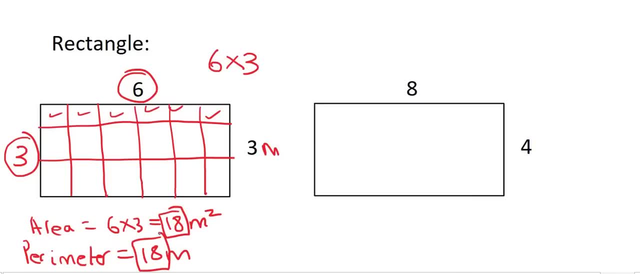 Don't worry about the fact that these are both 18.. That sometimes happens, but it doesn't always happen. Okay, moving on to the example on the right hand side. Well, this is very easy. We know how to do this by now. So, if we're to go work out the perimeter, 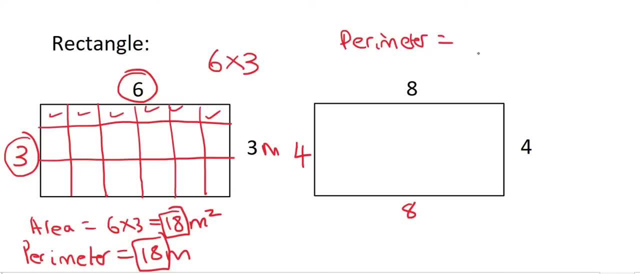 you would just say eight plus eight plus four plus four And that's going to give you 24 meters. then for the area we know that that's just eight multiplied by four And that's going to give us 32 meters squared. So you can see the way to work. 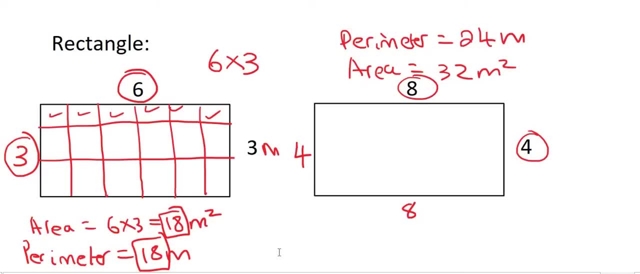 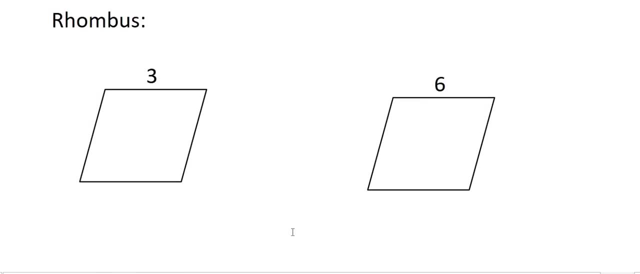 out the area and the perimeter of a square and a rectangle is pretty much the same. Now, moving on to a rhombus, which is like a square, but it's been moved over to the side. Now, if we were to go work out the perimeter of a square, we would just say eight plus eight plus four. 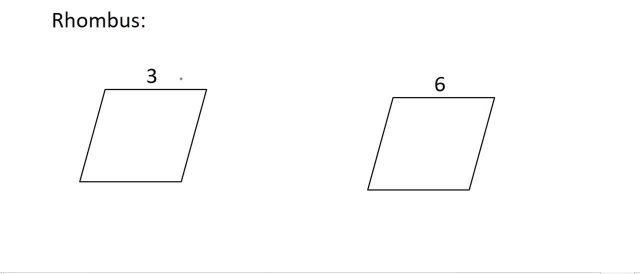 Now, because it's the same as a square that's just been moved over. all of the lengths of a rhombus are the same. That's something important you need to know. Write it down on a piece of paper. put it on. 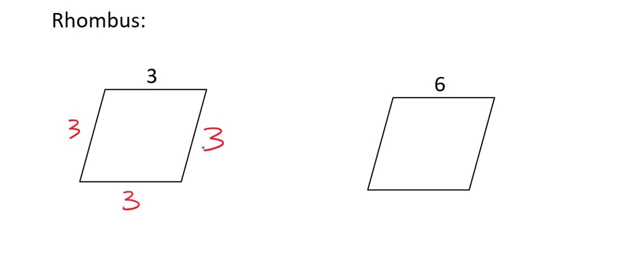 your wall in your bedroom. look at it every day so that you don't forget these different properties. Rectangles and squares are easy, but as we start getting to a rhombus it starts getting a little bit more difficult to remember. So to work out the perimeter, that's very easy. Three plus three. 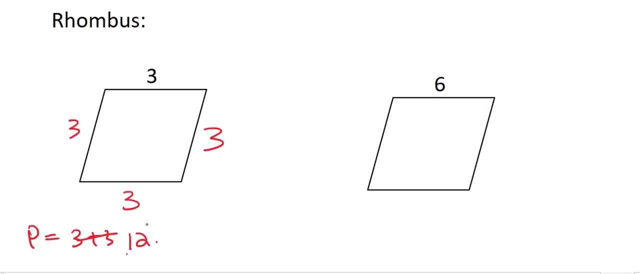 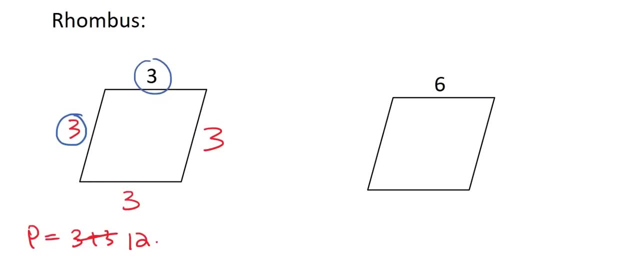 a rectangle, we would have just said three times three, But this shape is a little bit skew, It's tilted, and so we're not going to do that. What we need for a rhombus is the height. Now you might. 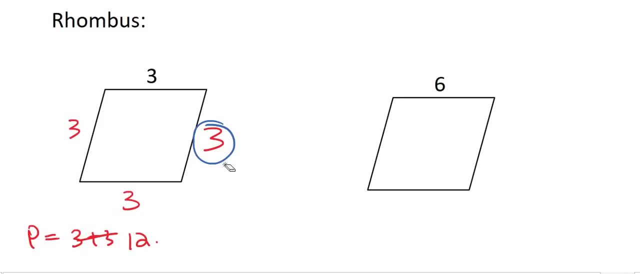 be saying, Kevin, the height is three. No, it's not. That height is not three. The height is this part over here, You see, from the top straight down to the bottom. It mustn't go like this, at an angle. We don't want that height, We want the height from the top to the bottom. And so they 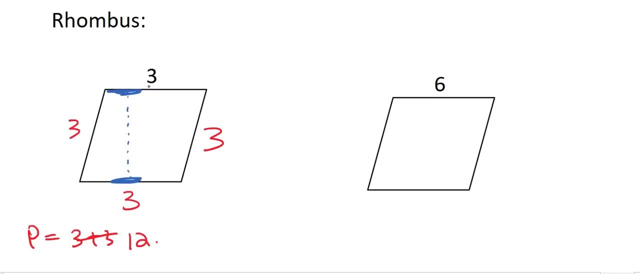 would have to give you that length, or somehow you would be able to work it out using Pythagoras, which I'll show you in videos later on. And so let's say, this length is two. So then to work out the area of a rhombus. now, this is important, guys, Pay attention, It's the base length times by: 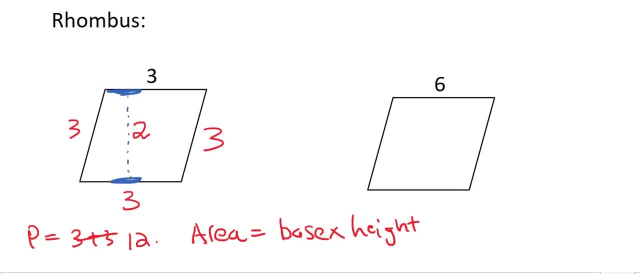 the height, And so the base, for example, could be three and the height is the two. The height is not the three, okay, It must be the base, and the height must be 90 degrees to each other. See that, 90 degrees to each other, okay, And so that's going to be three times two, which is 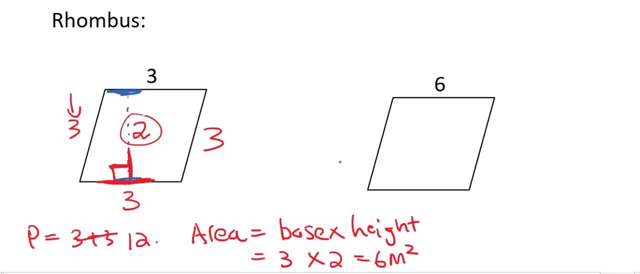 six, And let's say it was meters, So it would be meters to the power of two. So, moving on to this example, here on the right-hand side we've got, we know that it's a rhombus, and so all four sides. 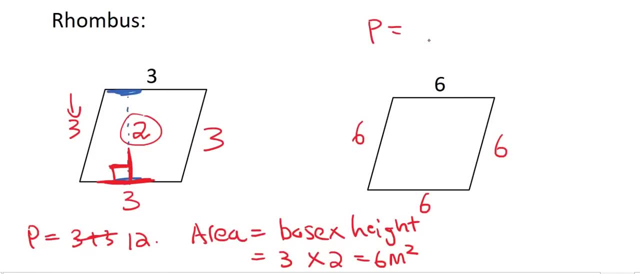 must be the same, And so to work out the perimeter, you could just say six plus six plus six plus six, or you could say six times four, and that's going to give you 24 meters. Let's say that it was in. 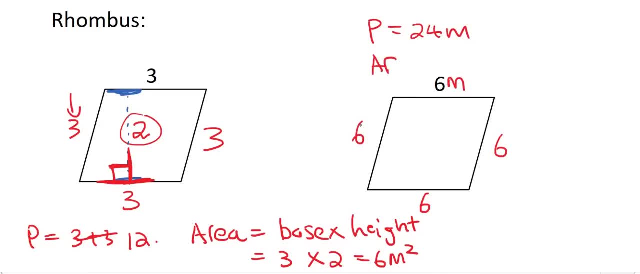 meters, Then the area is not going to be six times six. Please remember that, guys. Your area must always be from the top straight down to the bottom. Sometimes in a test, they'll even give you the height. like this, They'll give it to you on the outside of the. 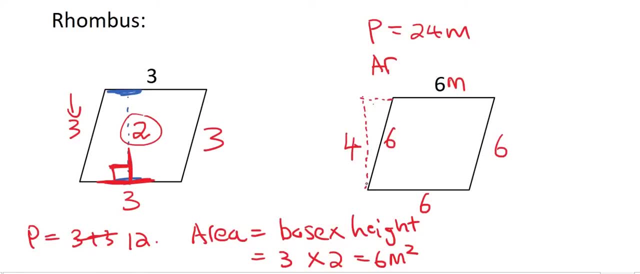 shape as a dotted line And some students, they're like Kevin. how can they give us the height if it's on the outside of the shape? Guys, it doesn't matter if this four is over here or if I show you. 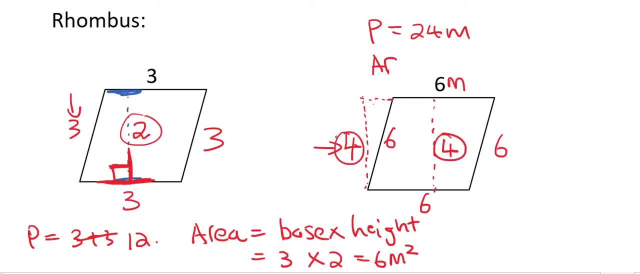 over here. these two would be the same height, okay, And so the area of that shape would be six times four, which is 24 meters squared. And once again, don't worry about the fact that these two numbers are the same. That sometimes happens, but most times it. 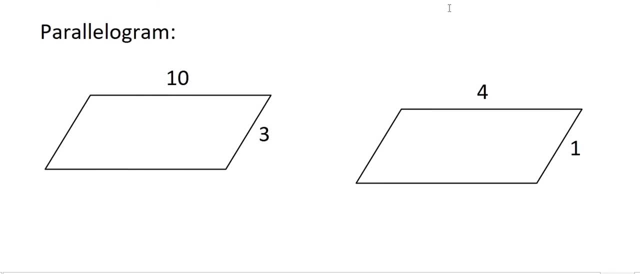 doesn't Moving on to the last shape for this lesson and that is the parallelogram. So the parallelogram is like a rhombus mixed with a rectangle. So the rhombus part- I say that because it's tilted to the side- but then the rectangle part is because it's tilted to the side, And so 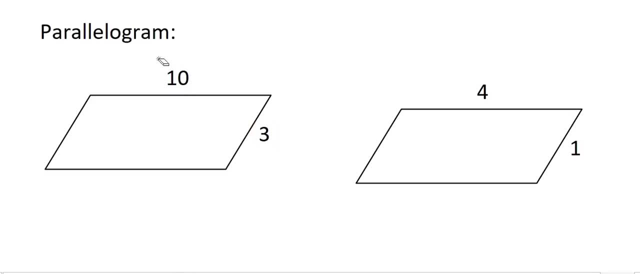 this whole piece here is the same as the first one, but it has a different length. It has a different shape and I'm going to use the base length as the base. okay, The base is going to be the same length because the lengths are different. Now, with a parallelogram, the opposite sides have the same. 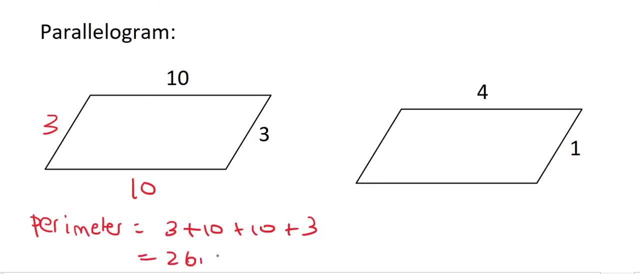 length. okay, And so to work out the perimeter, super easy, right? That's going to be three plus ten plus ten plus three, And that's going to give us 26 meters. To work out the area, once again, we're going to use the base length multiplied by the height. And remember, the height never looks like that, The height never. 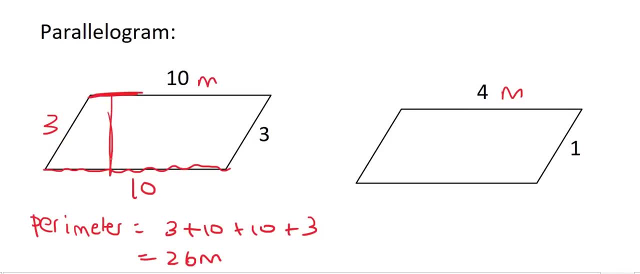 is always from the top down to the bottom, like that, as a straight or, and it must always make 90 degrees with your base. and so let's say that that length is 2, so the area is going to be the base length, which is 10 multiplied by the. 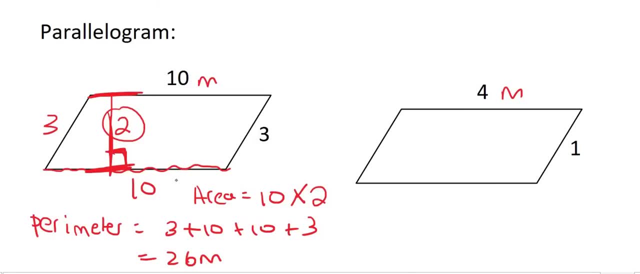 height length, which is 2, and, guys, when you use the base length, you could have even used this 10 up here. it doesn't have to be the one at the bottom, okay, and so that would give us 20 meters squared. moving on to the last little. 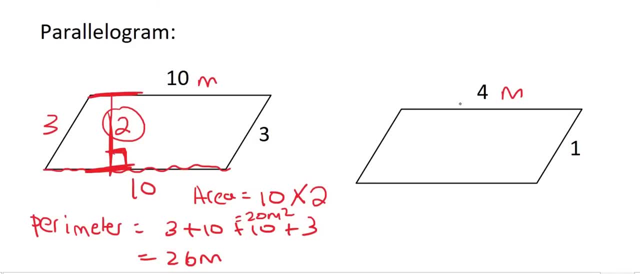 part of today's lesson, or this lesson. sorry you might be watching more than one. let's look at the perimeter. so for the perimeter, that's gonna be 4 plus 1 plus 4 plus 1, because this side over here is 4 and this side over here is 1. 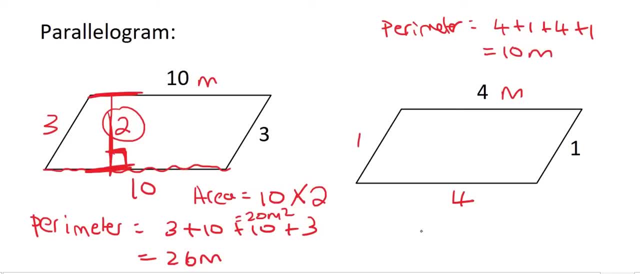 and if you go add that up, you're gonna get 10 meters. then, to work out the area, we would need the base length, which is 4, that's this one, but then you would need the height, and so they would either give it to you, maybe like this, and they'll say that: 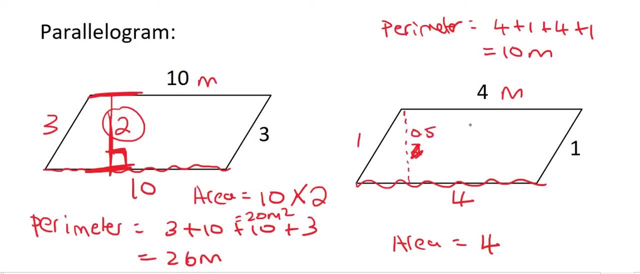 that's a 2. no, not a 2, it would be like 0,5, and they'll give you this one, maybe, or they'll give it to you over here or, as we said in the previous example, they could even give it to you on the outside, as long as it's going from the top. 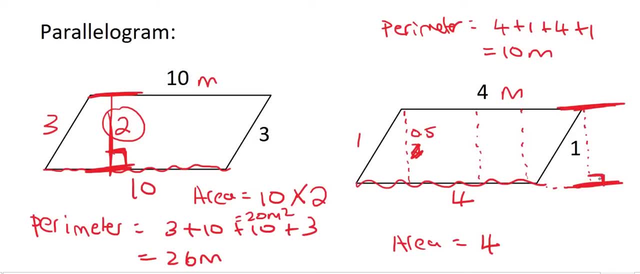 straight down to the bottom where it's making a 90 degree angle with the bottom, like that, or with the top. okay, can you see that? and so let's say that the height is 0.5, and so you suspect 4 times 0.5, and that would give you 2 meters squared, so in 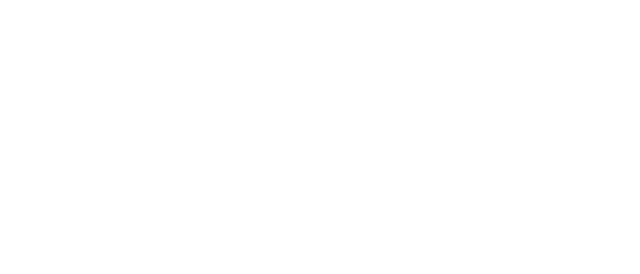 summary, the main things that I want you to remember from this lesson is that the perimeter is, on the outside now, 4 square. the area is always going to be this one multiplied by this one. so you just multiply the two sides together for a rectangle and notice here you wouldn't. 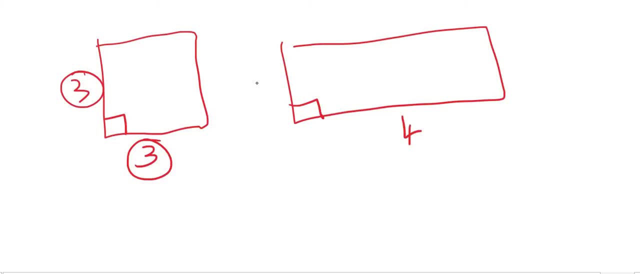 notice that that's 90. For a rectangle it's also 90 degrees, And so you just multiply the 4 and the 3.. But then when we start getting to shapes that are slanted or like going off to the side, like